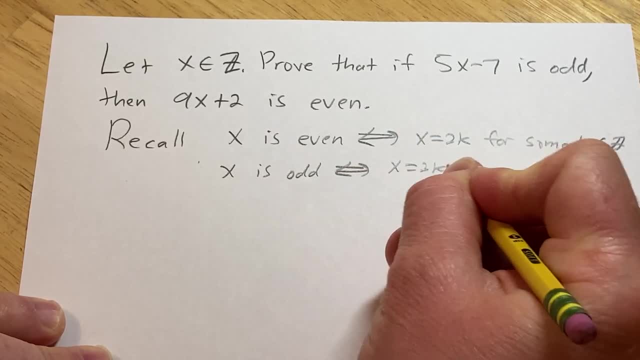 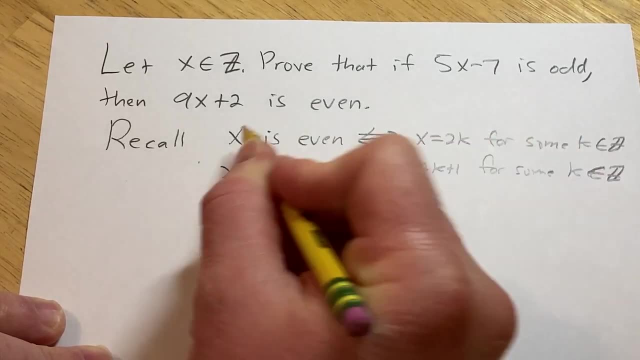 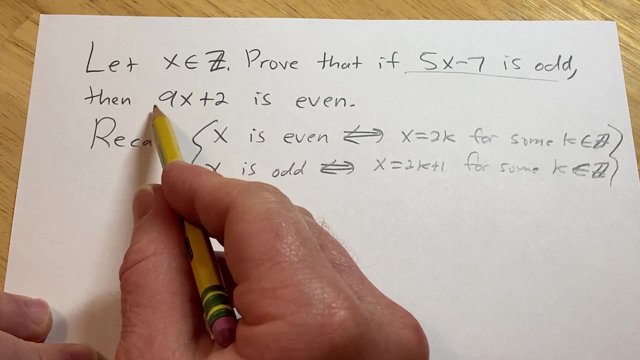 that's the same thing as saying: x equals 2k plus 1 for some integer k. So you have to know these cold in order to do problems like this. All right, we're just going to give a direct proof. We're going to assume that this is odd and we're going to try to show that this is even So. we're going to hold the proof line constant at x. Next, let me give you some인지. The first thing that comes in here that's going to dat for constant x is the value of theípite protection set. Let me give you another example. So we had this problem with our other identifiers. All right, 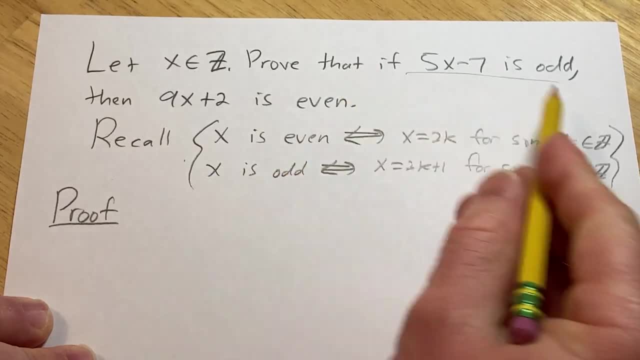 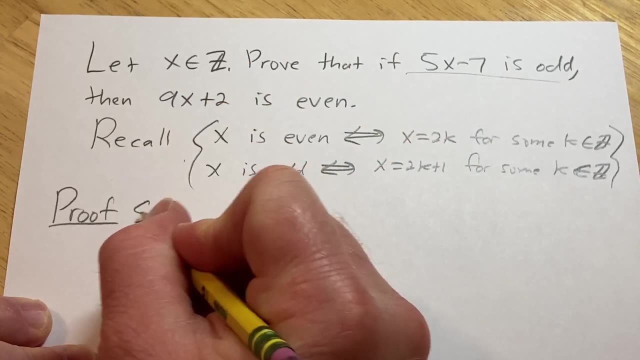 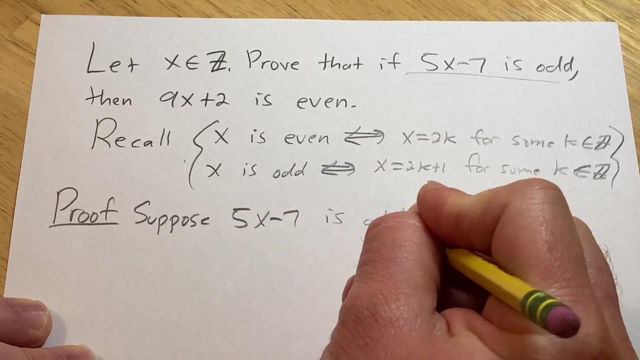 proof. so this is an if-then proof. so basically you assume this is true and then you have to show this is true. so you start by writing down your assumptions. so you say, suppose 5x minus 7 is odd, and then typically in these problems what you do is you write down what it means. what does your assumption? 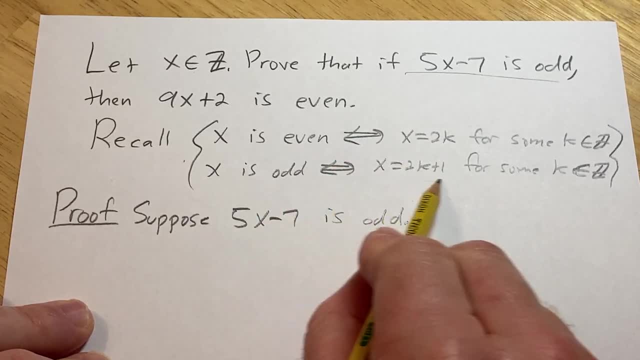 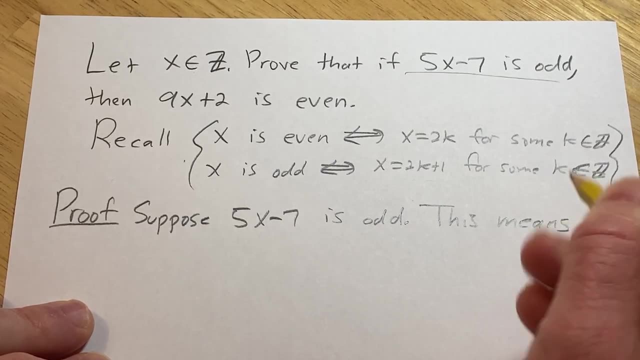 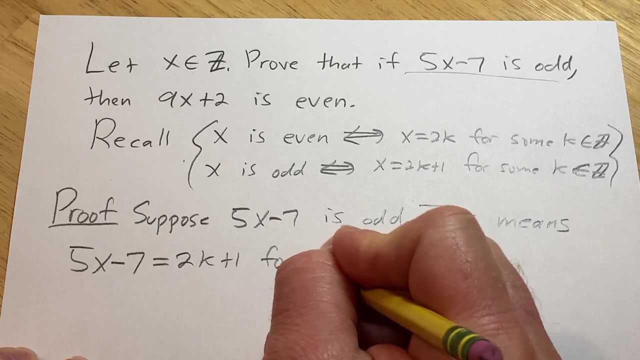 mean? so what does it mean to be odd? well, it means we can write it as 2k plus 1 for some k and z. so this means- and it even helps to write that you know this means 5x minus 7 is equal to 2k plus 1 for some k in the set of integers. okay, 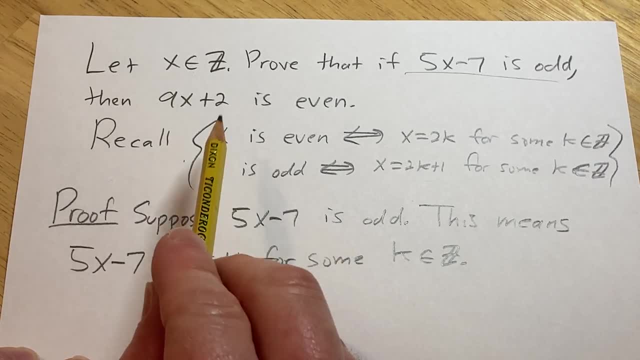 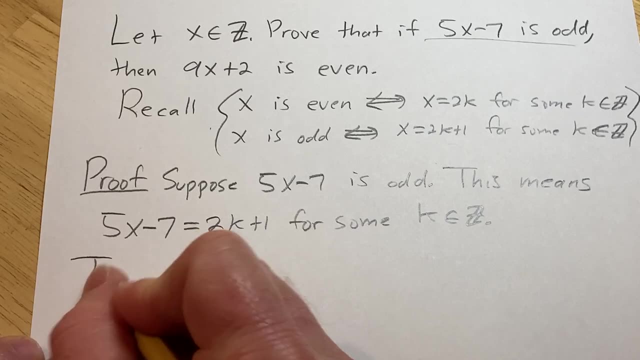 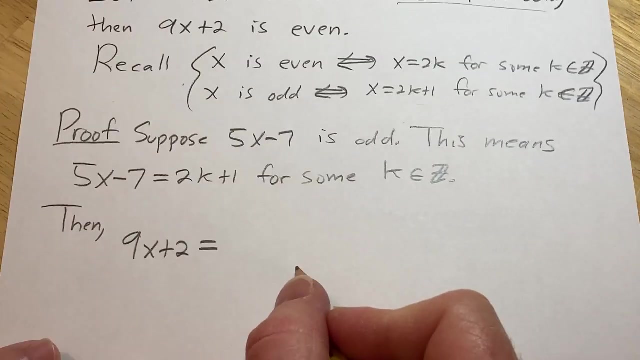 so now we have to look at 9x plus 2 and we somehow have to involve this, so let's see if we can do that. so then 9x plus 2 is equal to: so what I'm going to do now is something really clever, and 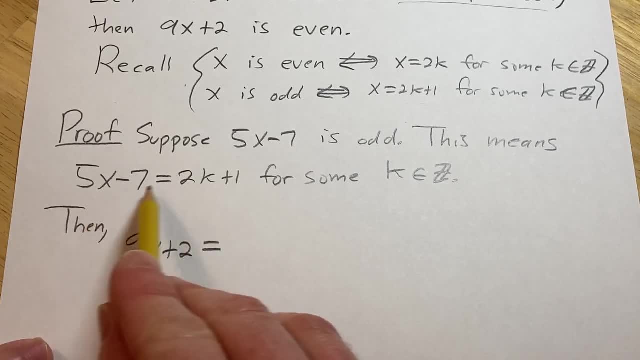 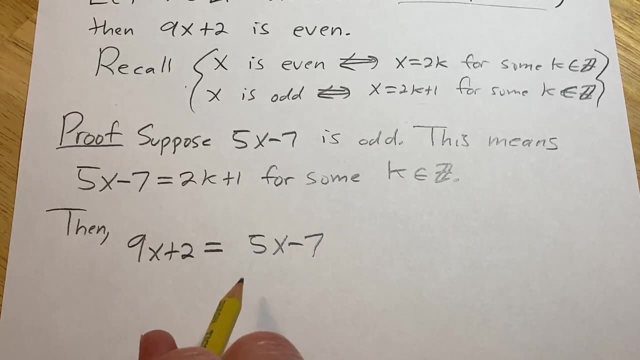 I haven't done this problem yet, but I'm just going to somehow involve 5x minus 7. to do that, I'm just going to write it down. so this equation is obviously not true. so in order to make it true, we need to make it true. so we have a 5x here. but 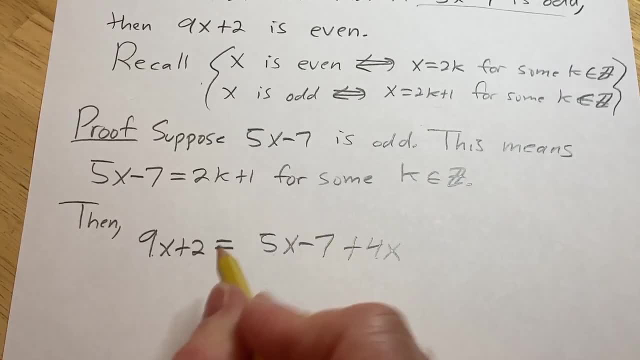 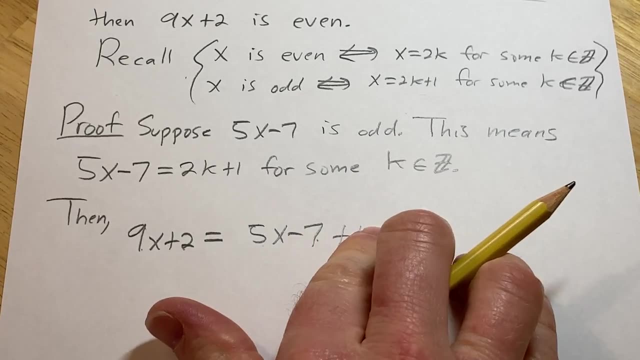 we need a 9x, so I can add 4x to this. we have a plus 2 here, but here we have a minus 7, so we need to make it true. so we need to make it true. so we have a 9x, so I can add 9 to this. let's check that. so, again, I wrote down what I wanted. 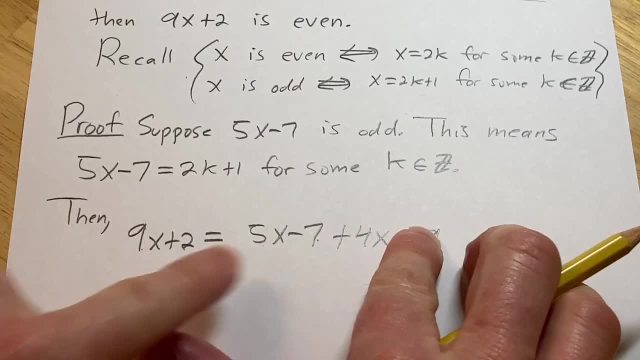 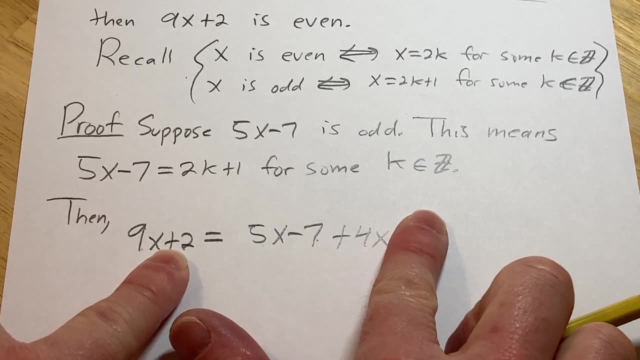 I say, hey, I want a 9x, I want it to be true, so I'm going to put a 4x here. 4x plus 5x is 9x. hey, I want this to be a plus 2, but I have a minus 7, so I'll put: